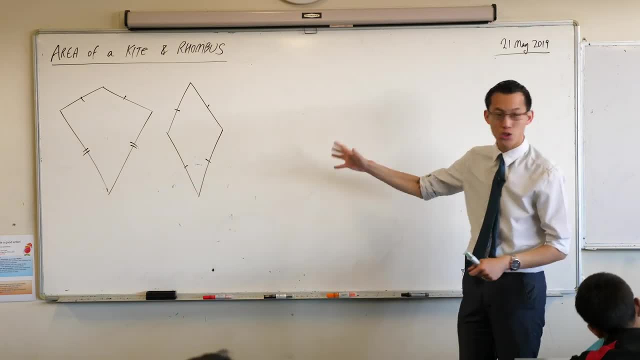 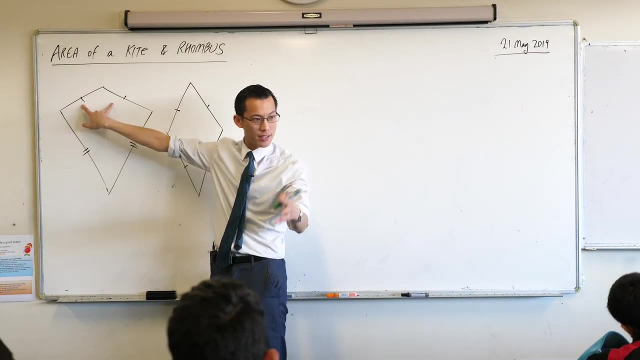 So when you take a kite or a rhombus, just draw it up. Remember, the key feature of a kite is that you've got these two sides being the same, adjacent sides being equal in length and these two also being equal. 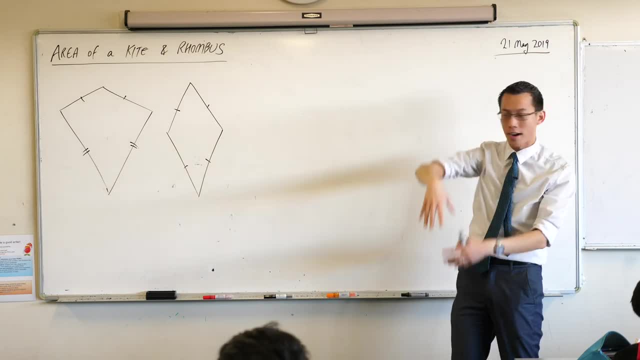 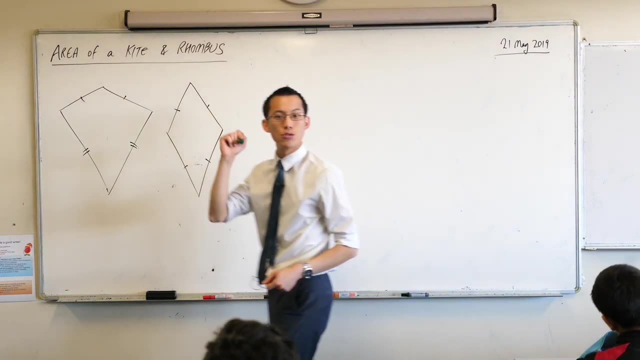 If you took those two pairs and made them equal to each other, then you'd end up with a rhombus. All four sides are equal in length. What I'd like us to do is to draw the diagonals of these two shapes. 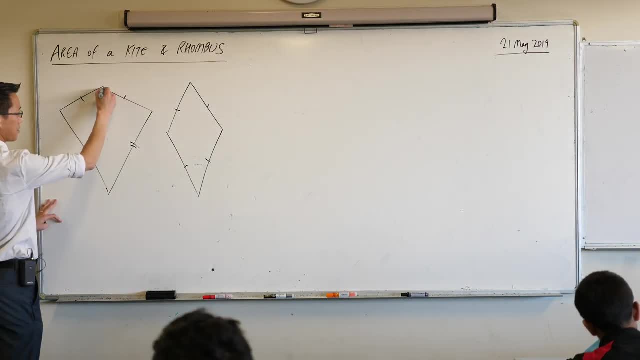 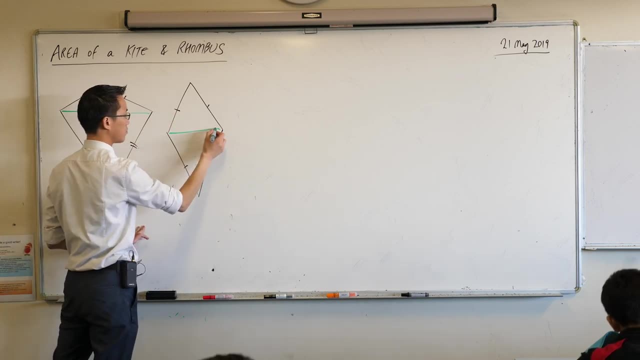 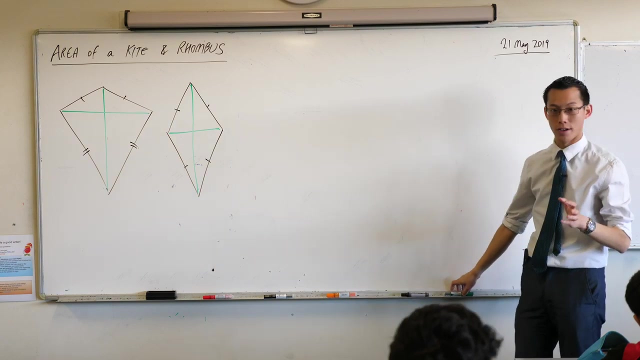 Can we please draw the diagonals of these two shapes? Now, if you have actually used a ruler and you've drawn your kite, it's actually a kite, like you've measured out. You've drawn your rhombus: It's actually a rhombus. 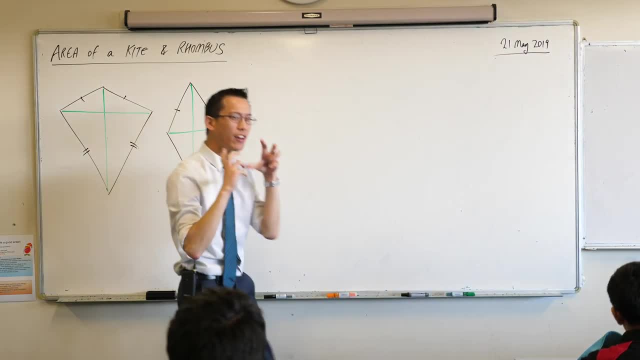 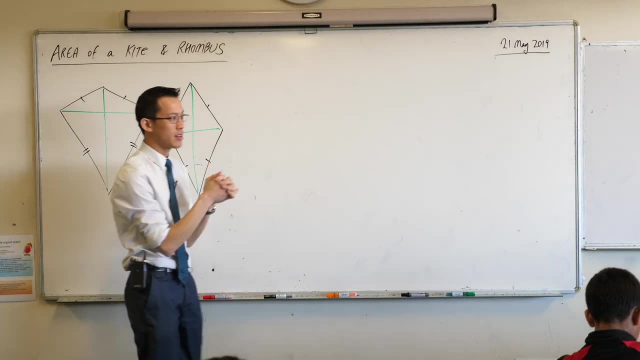 Every side matches. Then when you draw your diagonals, you cannot help but notice that the diagonals have this nice, peculiar relationship with each other. They meet at a certain angle. Can anyone tell me what that angle is? Say Hindu. 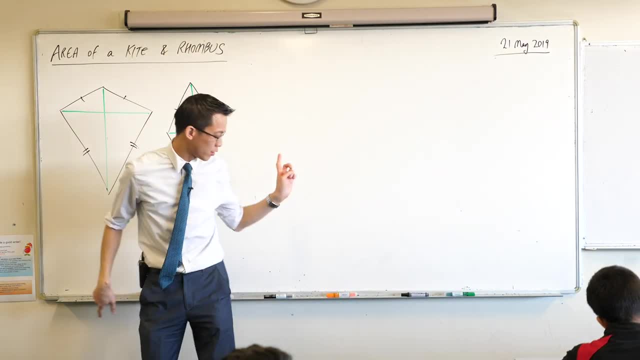 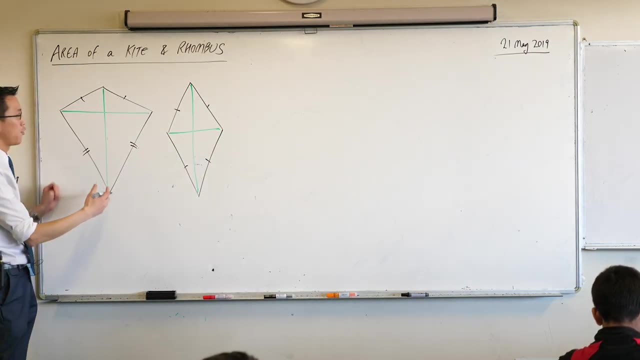 It's 90 degrees, right? So we would say: these diagonals are what's the word when two things are 90 degrees? Yeah, Hindu Perpendicular. Thank you very much. Can you please indicate for me this is perpendicular and this is perpendicular. 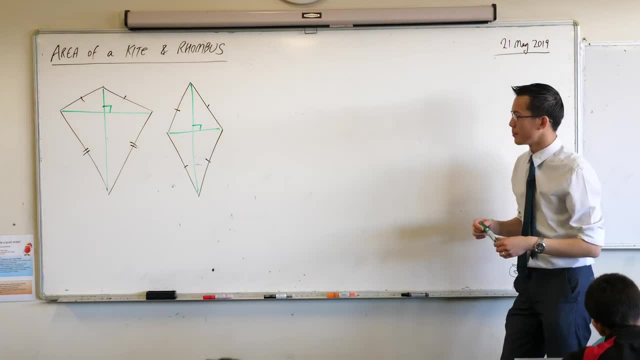 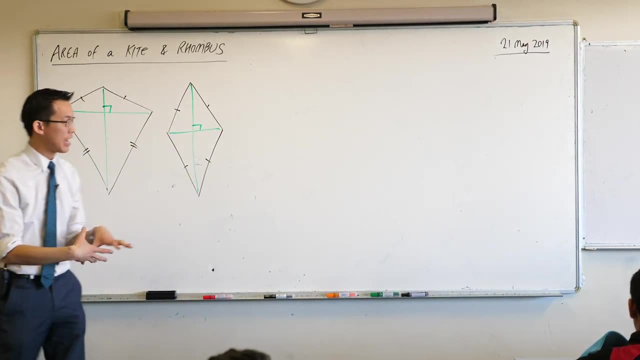 Okay, So we've got our right angles. Now remember when we had a look yesterday. you can take a shape like a trapezium and you can cut it up, you can rearrange it so that you get a shape that's easier to calculate. 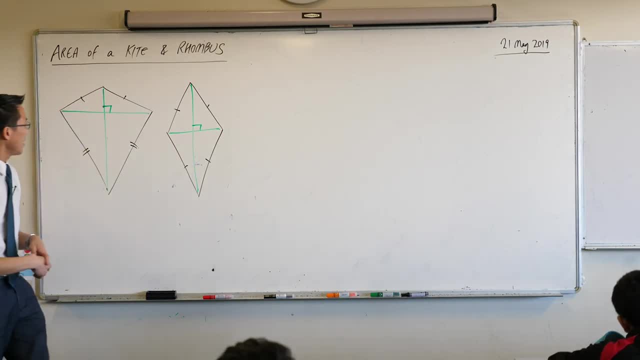 We're going to do the same thing here. We're going to do it twice. Have a look over here. Let's look at the kite right? Do you notice the kite has a kind of symmetry. Do you see that It's symmetrical, like these guys are the same and these guys are the same, right. 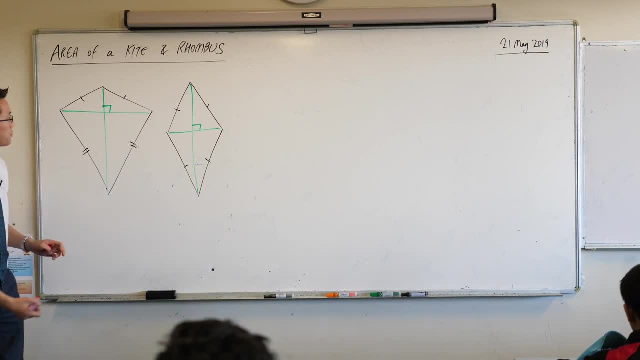 So what I want you to, if you can, if you've got another color, that would be enormously helpful. What I'd like you to shade in with me is that these four triangles here are not actually four triangles, it's two triangles done twice. 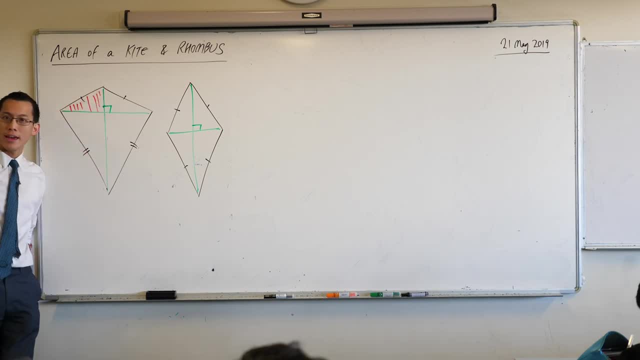 See this guy over here. I'm going to shade this one up the top in red. This red triangle is identical to this red triangle. Can you see that? They just mirror images of each other And it's the same deal with the ones on the bottom. 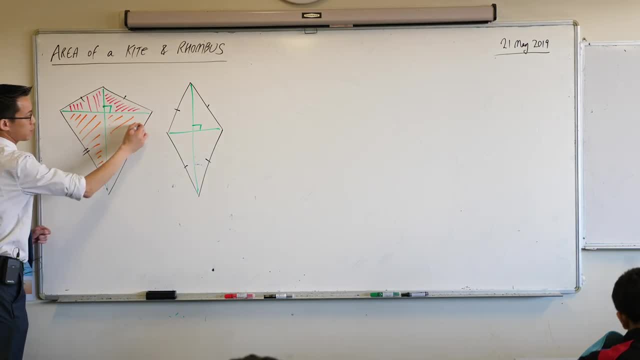 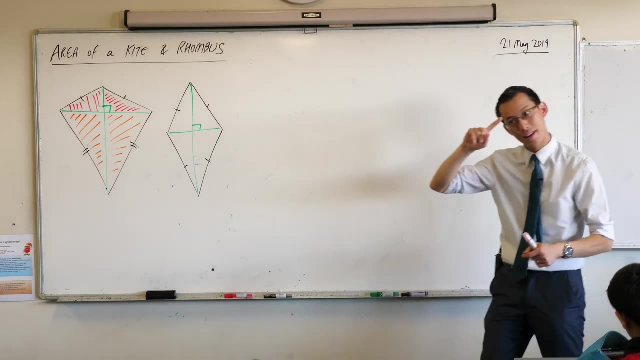 These two triangles here are equal to these two triangles here. Okay, Same for this, which we're going to deal with a little more next year, But I'm going to tell you what the word is now, so that in 12 months time you're like: 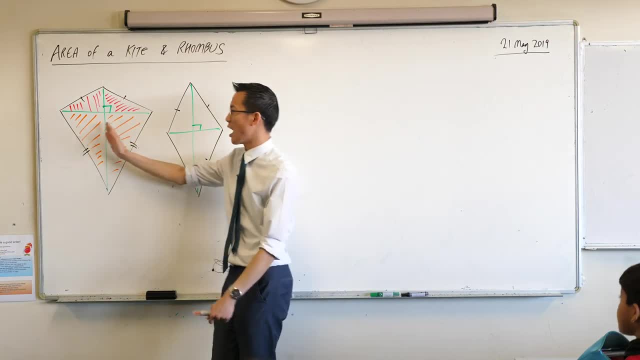 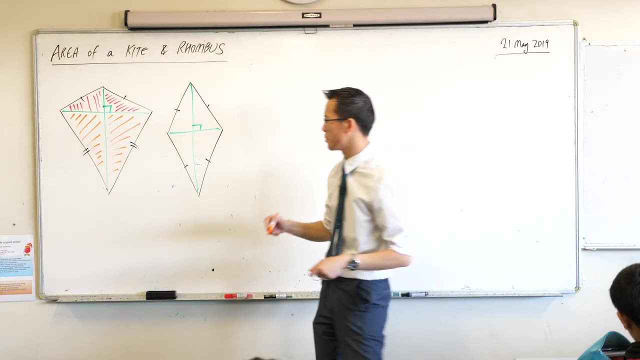 ooh, remember that thing Mr Wu said: When these triangles are the same in every single way, they're the same size, same dimensions. all that we call them congruent. Congruent, It's a bit of a funny kind of word. 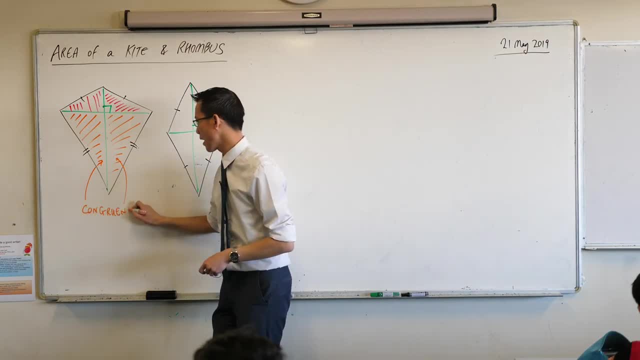 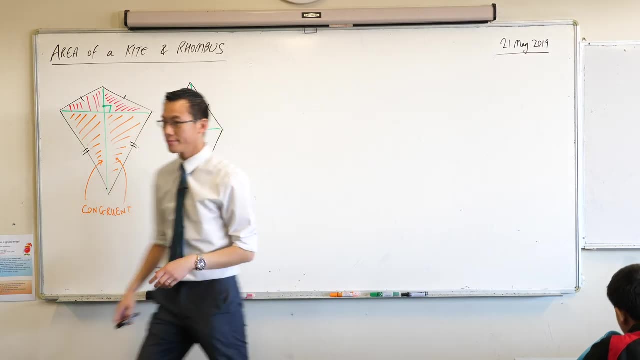 Here's how you spell it: C-O-N-G-R-U-E-N-T. They're congruent, identical in every way, including their area. So what we can do is, if you'd like, just eyes up for a second and watch this part. 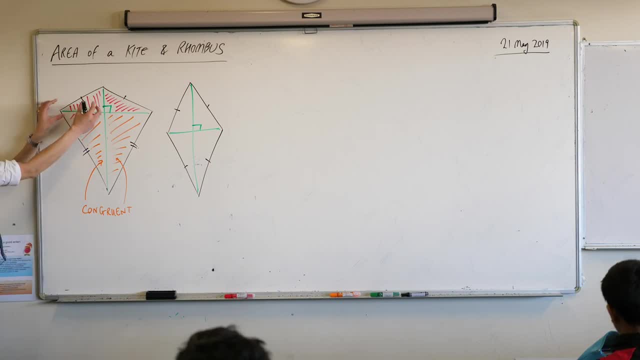 You can then go back to doing your own drawing. Imagine taking this red triangle here and ripping it off and then spinning it around so it'd fit over here. Can you see it would fit in nicely on that corner. Can you do that? 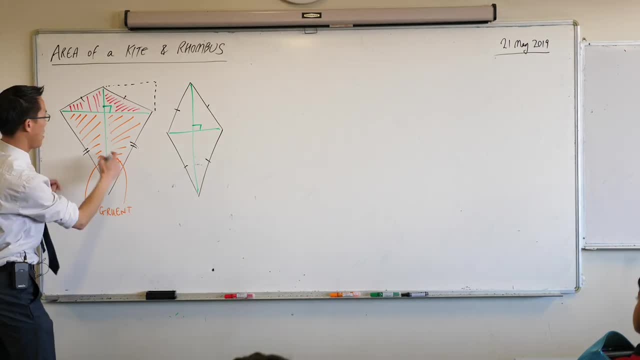 You can do it on your own and you can match it with this orange one down the bottom. I could take this left-hand triangle, sort of rip it off and then spin it around so it fits over here. Okay, So now. 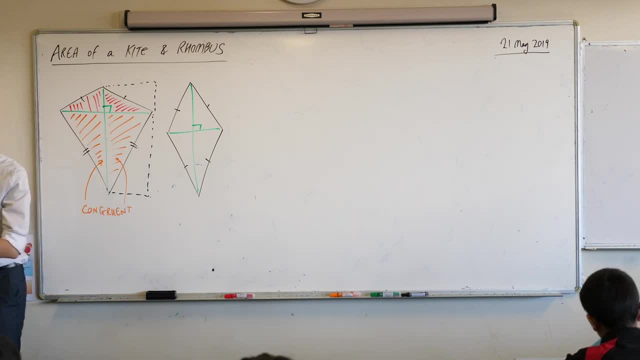 having moved this shape over here, I'm just going to do my very best with this poster. Perfect, Okay. What shape is that? That's a rectangle, right. All we need is its base and its height, and we're there. 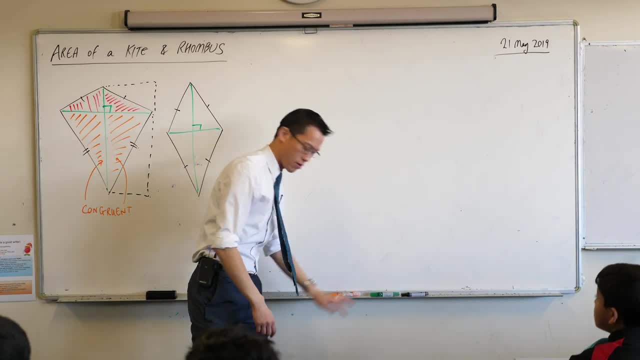 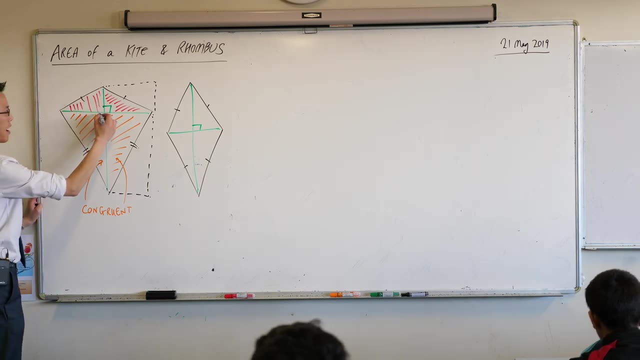 Okay, So in a kite or in a- Where'd my black one go? Here it is. Or in a rhombus. we usually call these two diagonals X and Y. So if I put an X All the way across there and a Y which goes all the way up and down, 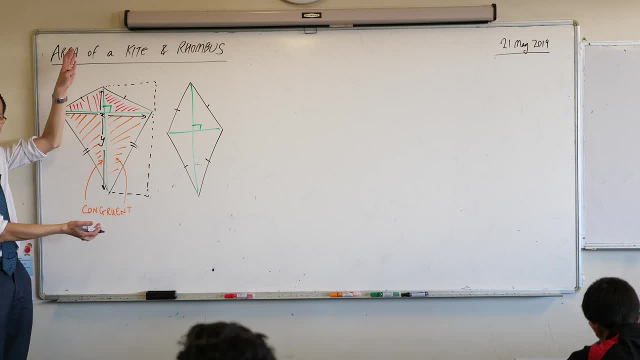 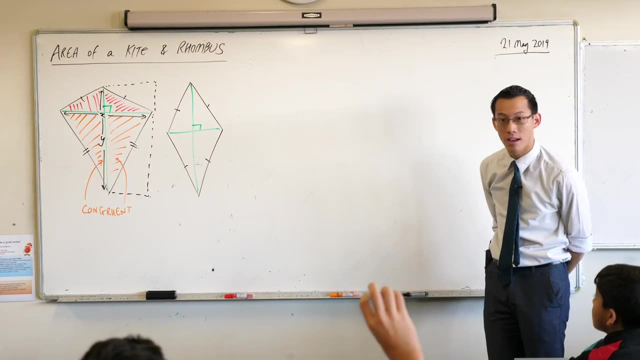 What is the height of the rectangle that we've drawn? Not a rhetorical question, it's just very straightforward. The new rectangle on the right-hand side. how tall is it? Have a look, Krishan. what do you see? Y times, half of X. 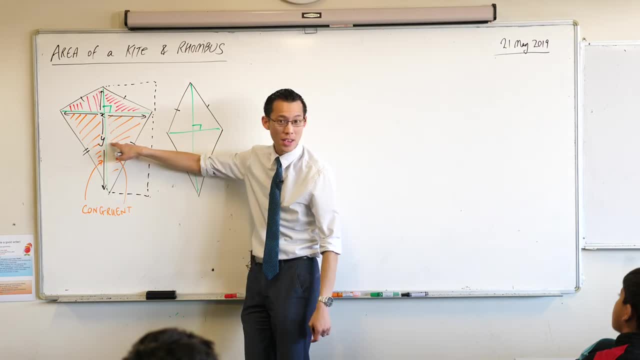 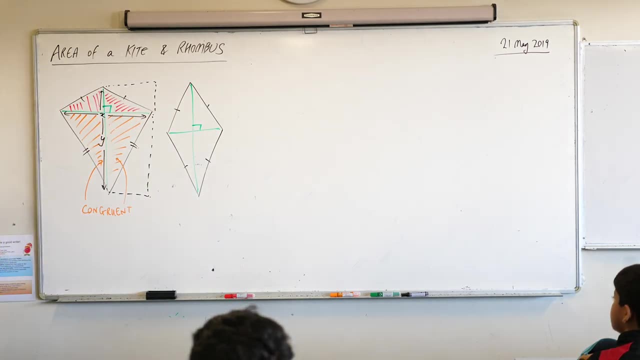 Ah, okay, so you've already gone to the next step, haven't you? The height is Y. Where did you get? Where did Krishan get half of X from? Where is that Here? where do you see it? Because you see the diagonal. 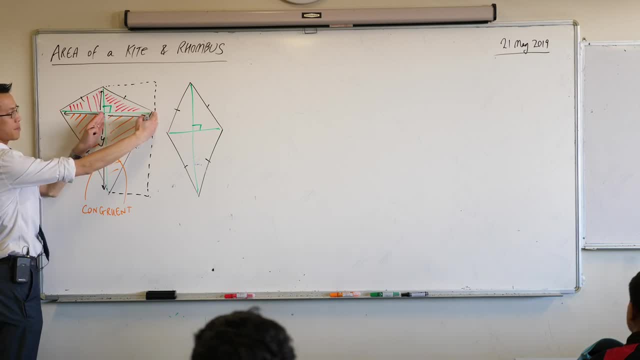 Because you took off that piece and the other piece. Yep, Very good. So we've got this rectangle. it's half Sorry, it's Y, all the way from the top to the bottom. And then, when you have a look at this rectangle,